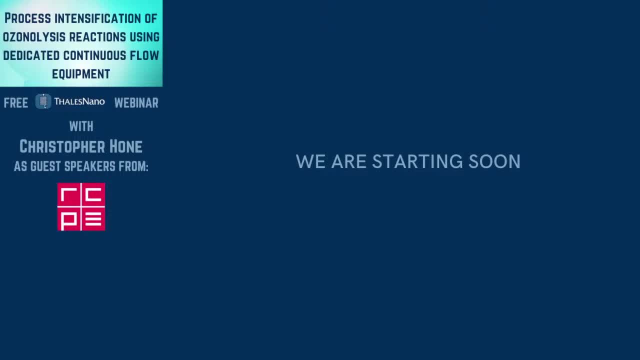 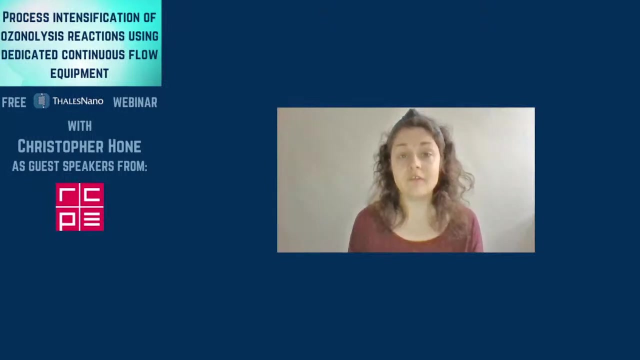 Thank you, Thank you. Thank you everyone on today's webinar, which will be held by Christopher Holm from the Center for Continuous Flow Synthesis and Processing from University of Graz, Austria. Today, he will talk about process intensification and ozonalysis reactions using dedicated continuous flow equipment which features Dallas Nanos Ozon module. 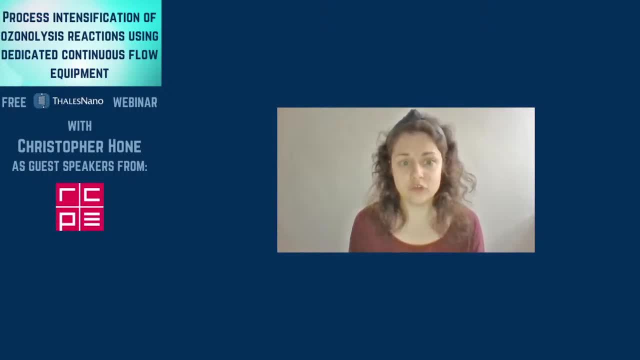 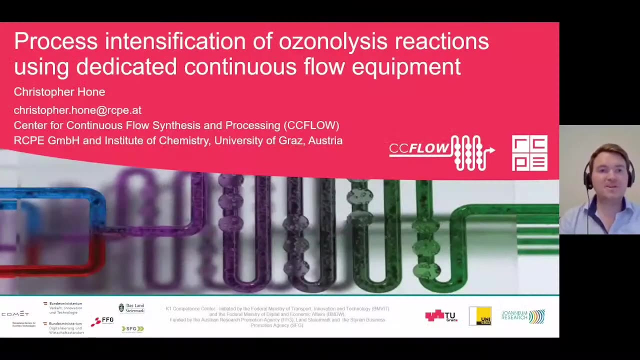 After the presentation, you will be able to ask your questions in the chat box or you can send them directly to us At askthechemist at dallasnanocom. Now let me hand you over to Christopher. Enjoy the presentation. Hello, welcome to today's webinar. I'm Christopher Holm. I'm from the Center for Continuous Flow, Synthesis and Processing- CCFlow- at the Research Center for Pharmaceutical Engineering. 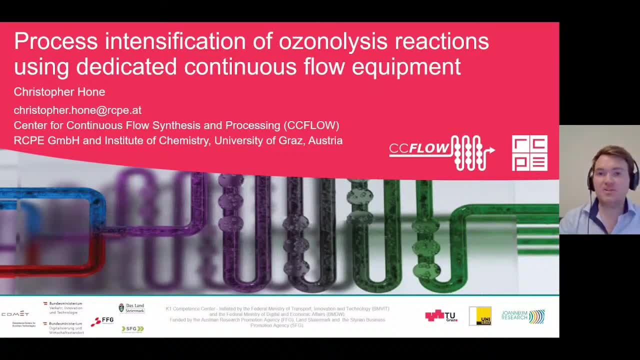 We're based in Graz in Austria, And today I'm going to be talking to you about the use of ozone as a reagent in organic synthesis And, in particular, ozonalysis reactions and how you can do them within continuous flow technologies. So I'll give you a general overview, to begin with, of this type of chemistry. 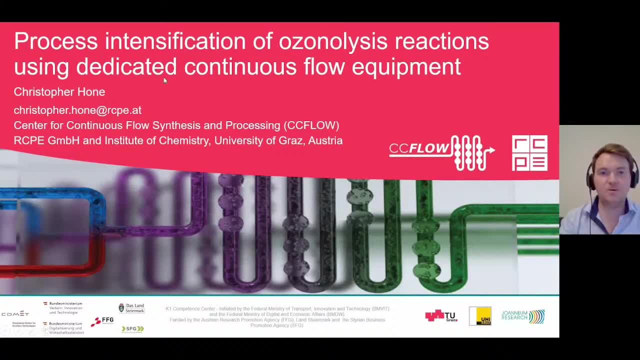 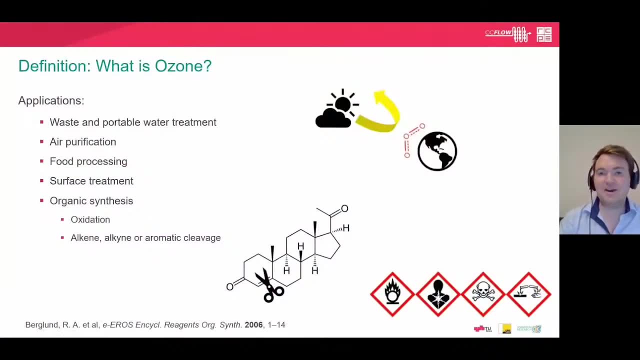 And then I'll talk more specifically about a research case from our group. So ozone is a naturally occurring molecule. It forms from molecular oxygen within the atmosphere by the action of ultraviolet light and electrical discharges. It's very unstable, and it also has many commercial applications as well, so many of which I'm sure you're familiar with. 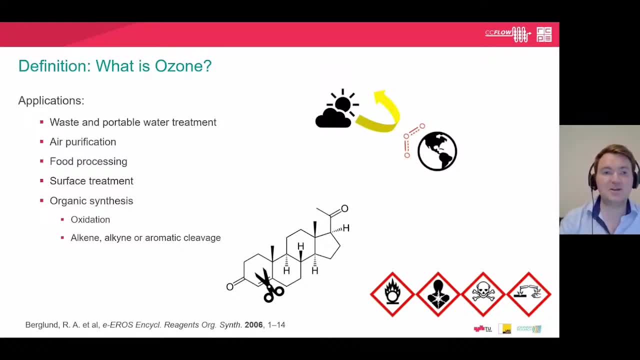 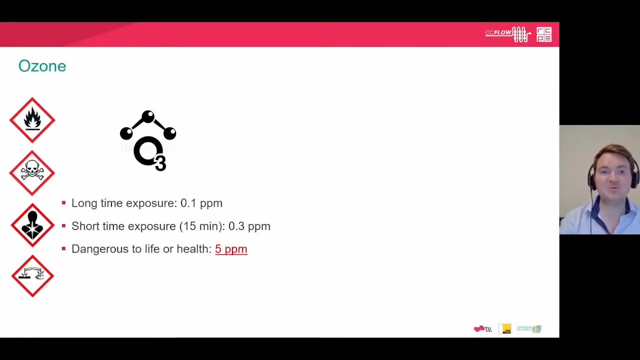 And the one that we're most interested in is naturally organic synthesis, so oxidation type chemistry, and also the use of ozone for performing alkyne and aromatic cleavage type reactions. So ozone itself it's got a bent type structure, so it's got a similar structure to water. 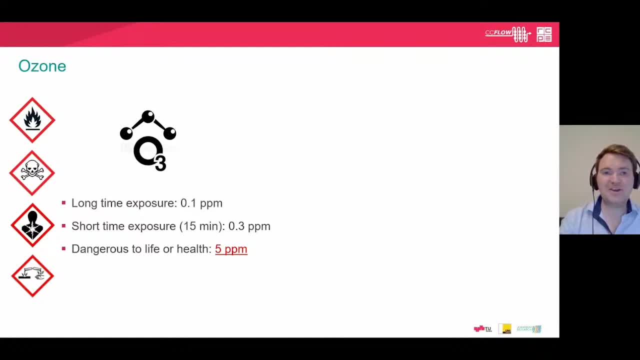 Ozone is a gas with a very pungent odor. it's pale blue in color, And one thing that I'm sure we all know about is it's a very toxic gas as well, so it's very dangerous to health, so it needs to be very carefully handled. 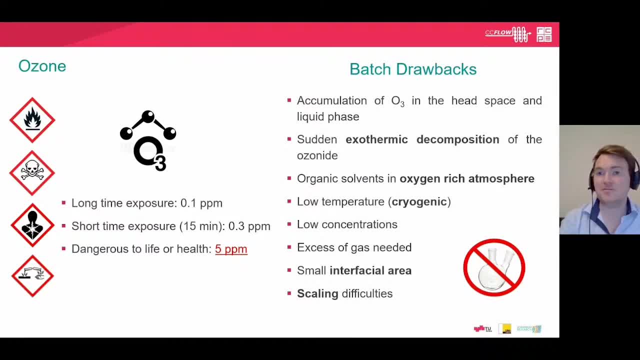 In terms of its drawbacks within batch vessels. So This sort of is that these are the drivers of why, then, we would want to perform this type of chemistry within continuous flow technologies is that the accumulation of ozone within the headspace and within the liquid phase of batch reactors is very dangerous. 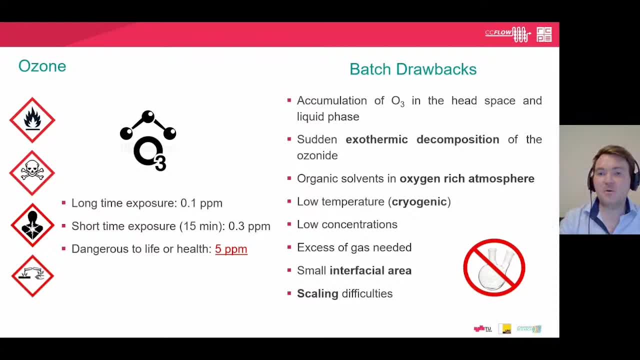 We also have the ozonide intermediate that forms with this chemistry that undergoes a very exothermic decomposition, So this needs to be very carefully controlled. We are operating with organic solvents and within these systems we have very oxygen rich atmospheres. so there's the potential for flammability because we need to carefully control the temperature. then we use cryogenic conditions which can be quite challenging to handle in terms of 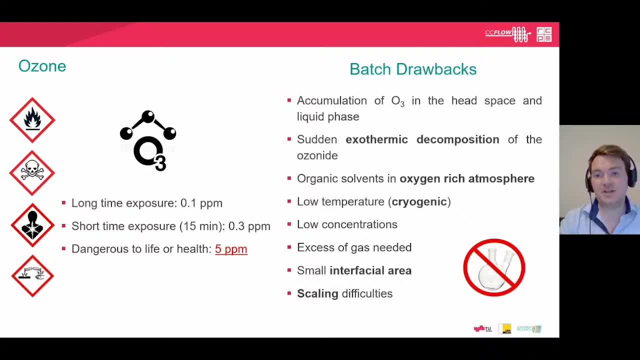 Accessing those lower temperatures, particularly at scale, because we want to try and minimize many of the exothermic intermediates. then we operate this type of chemistry at low concentrations. We also need an excess of gas, so this is quite inefficient, and then as we go to large scales we have quite a small interfacial area and then reactions can become mass transfer limited. 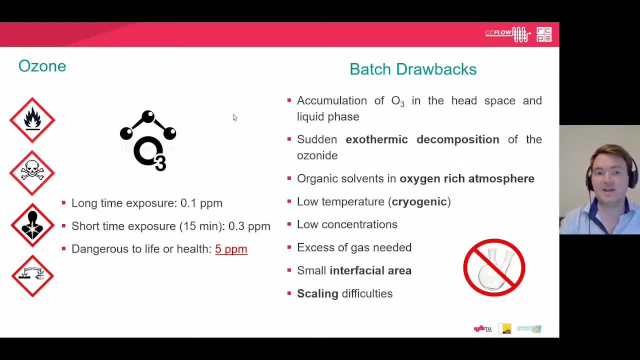 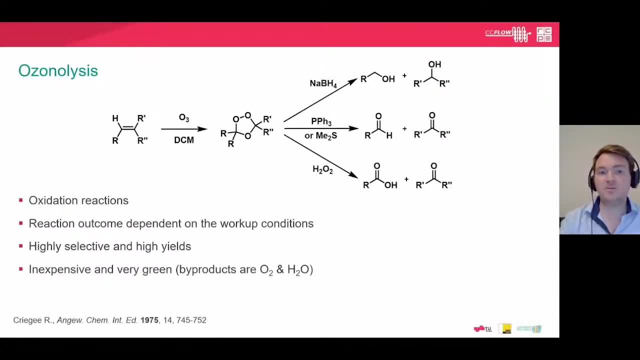 So all of these Aspects then clearly lead to scaling difficulties. So the type of chemistry that you can do, so at the top we have an alkene based reaction with ozone. And then the nice thing about this chemistry, depending on the quenching reagent use, so the work conditions, we can actually access quite a number of different products. so it gives us quite a 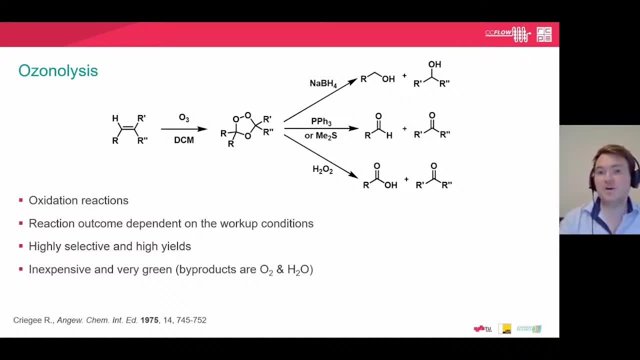 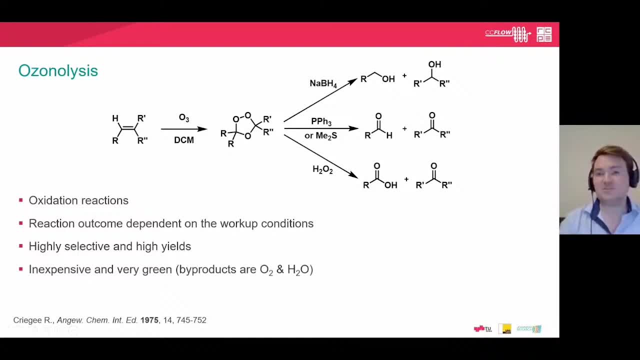 acids And in general. these reactions are quite highly selective and also provide high yield, and they are quite green as well in terms of that. the only stoichiometric byproducts that we form from these reactions are oxygen and water. So there are potential benefits, even though there 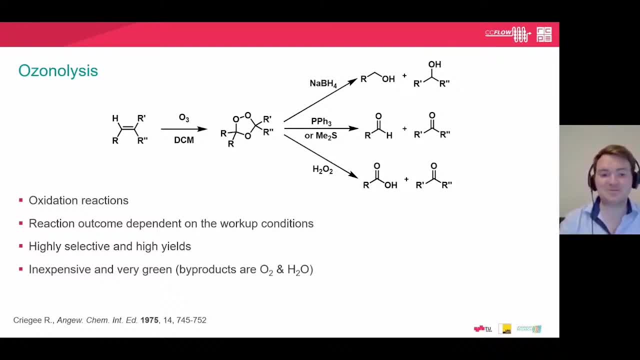 are limitations when it comes to handling the chemistry, in terms of the safety, And again, this is just a mechanism to show that, from the intermediate that we observe, then this can exothermically, this decomposition of this can be quite exothermic. So just turning now to give you 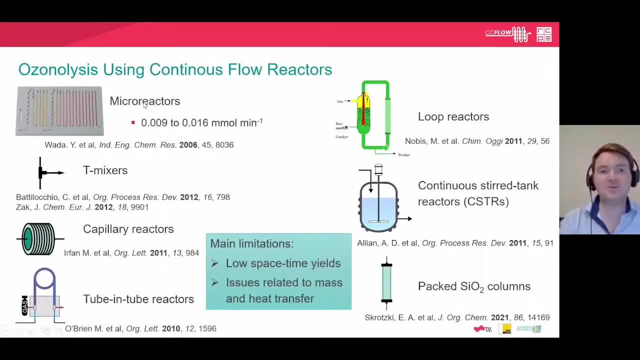 an overview of what's already been done within continuous flow. So the first example for it was from Jensen within a microreactor back in 2006.. So in this study they basically paved the way to show that it was possible to do this. Perhaps. 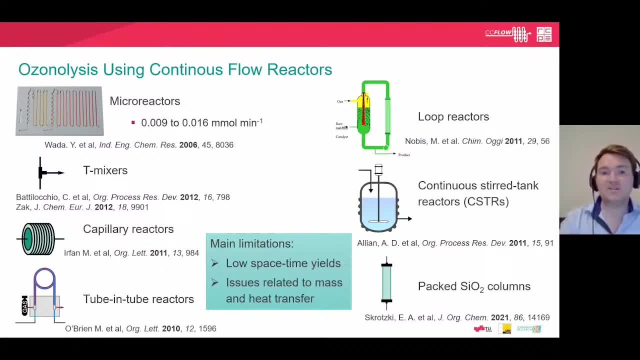 the main take-home message is that it's very difficult to achieve high throughputs within this type of system. Then subsequently, Stephen Lay's group looked at just using tea pieces for performing ozonolysis reactions, and this works very well because generally these reactions occur very quickly. So 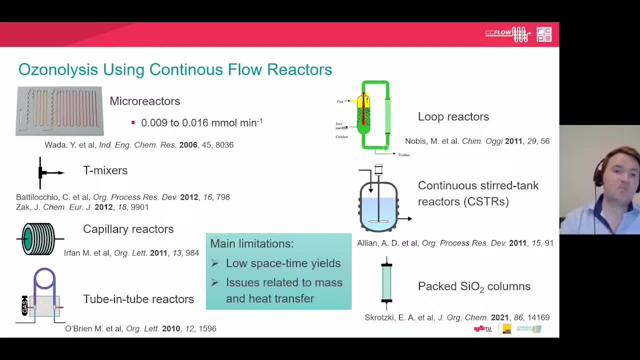 on the second to millisecond time scale. the problem comes is when you want to scale this chemistry up within a tea mixer. then you need larger diameters and it can be hard to predict how then the chemistry will perform at large scale and how the chemistry will perform at large scale. 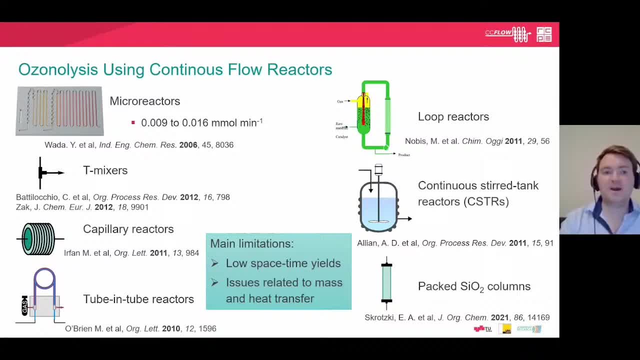 How do you thermally manage the system? Also an earlier example from our own group, using tubular capillary type reactors to perform this chemistry. again, this had the same limitation in terms of it was a relatively low throughput and it's very difficult scale from this kind of 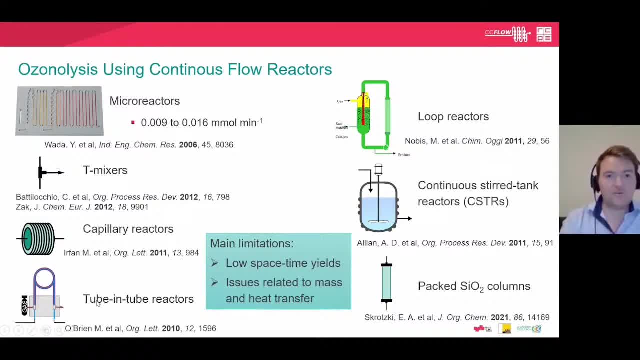 reactor for a gas liquid type reaction. Moving on reaction, And then Stephen Lay's group also reported the use of ozone within tubing tube reactors. This is a very interesting approach whereby there's a tube within a tube, with the middle tube is constructed of a semipermeable membrane which allows passage of the gas through. 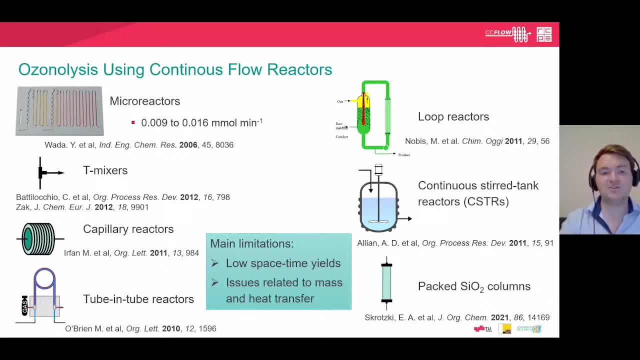 but doesn't allow passage of liquid. So it means you have your gas and your, you know, allows the passage of ozone through, which means that then you don't have a gas-liquid system within one compartment, So the ozone is all dissolved within the liquid phase. 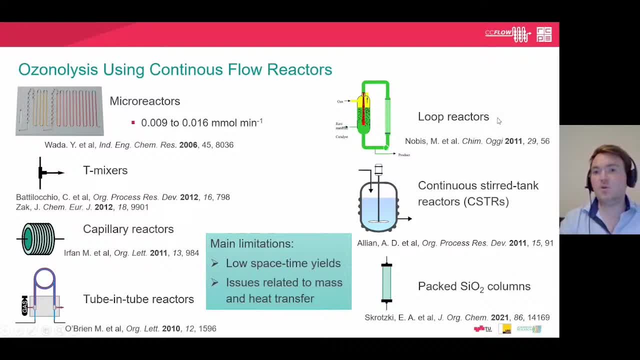 which makes it safer to handle. Also, loop reactors have been reported whereby the liquid feed is recirculated through the reactor. This can be quite useful for operation at scale. Continuous stirred tank reactors: again another solution for operating at scale. The ozone needs to. 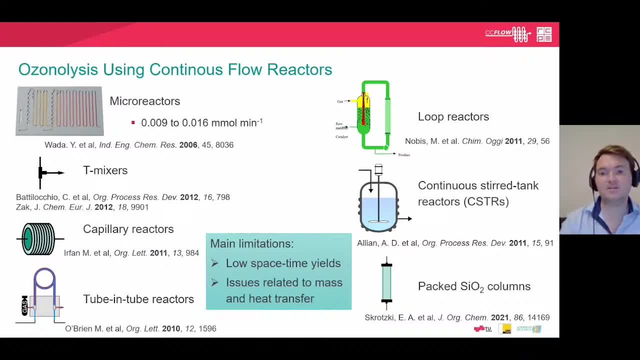 be carefully kept below certain levels. So that's a challenge, because a CSCR in some ways has similarities to batch-type reactors, but it does give the potential for scale-up by continuously throwing through your liquid feed And then, very recently, an approach. 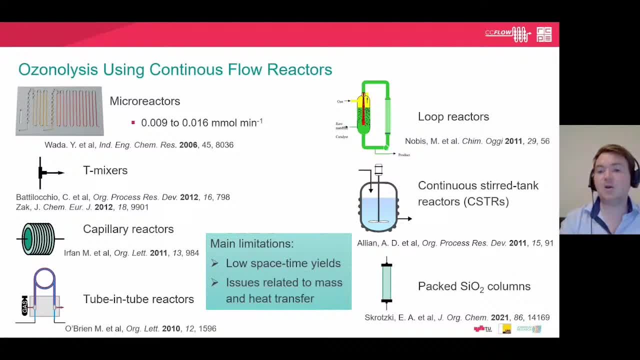 whereby silicon dioxide In part. in the most recent research, a graph showed thatylenol and other solvents and other compounds in a past life of a young man that so in recent lives carbongravity and acidity have increased, So it was not so easy to find out how this would be and is. 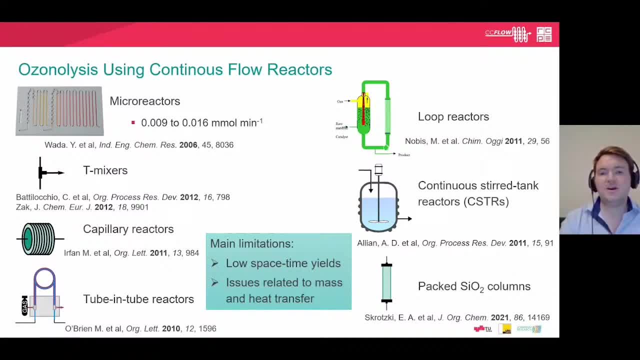 being studied. In the most recent research, we were able to find out that these compounds would kicked off the familiar cycle and weren't used to generate oxygen. Thus, we would be able to collect an amount of oxygen soon after the diffusion, And if you think you need to do this on a daily basis, then it is probably not that easy. 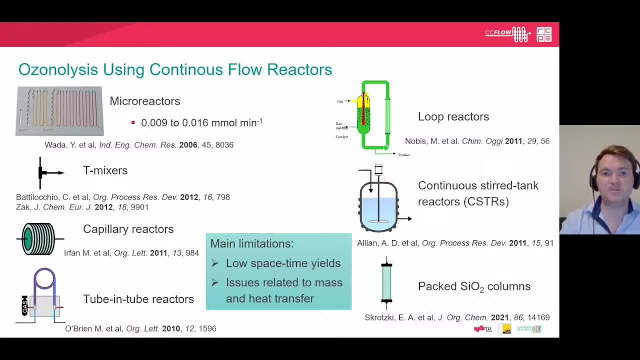 It's not like you should train in the kitchen to collect the oxygen. It's like you are in a webinar and you have to be in a restaurant where there is a kitchen and there's a kitchen where there is a kitchen clearly help in terms of scalability, but these are all excellent examples of how ozone has been. 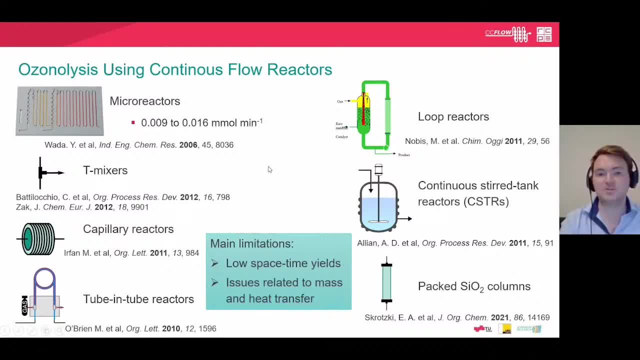 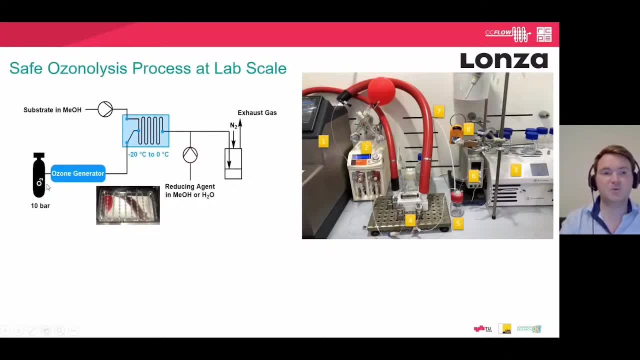 used as a reagent for organic reactions within continuous flow. So here is our general setup in terms of we have oxygen, which then passes through an ozone generator to form ozone, and we have our liquid feed, which is introduced via a pump and then this flows through a 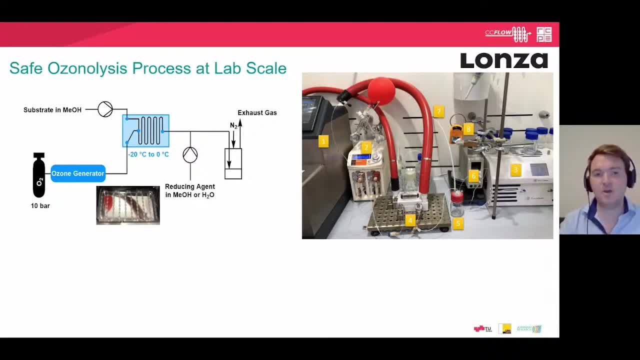 micro reactor, so in this case the lonzer flow plate manufactured from by Airfall, and then at the end of the reactor we have our quenching feed and then this flows into a vessel which has a nitrogen purge and an exhaust gas to ensure that we don't have high levels. 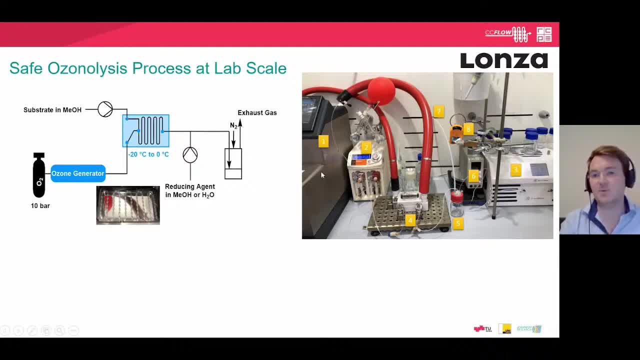 of oxygen in the engine and then this goes through a pump and then this flows through a liquid feed and it forward, and then this flows through a promoted liquid feed, which is a ratings undesired gas. so on the right hand side we have the set up as a picture in terms of having the 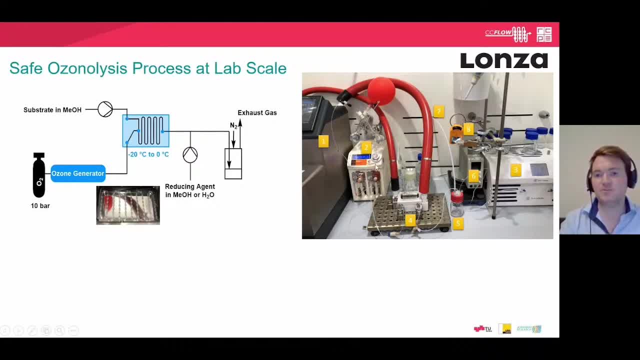 thermostat. we have a serious syringe pump for introduction of the liquid feed, the flow plate here. we have our outlet tube in here which has our vent and our um and our nitrogen purge, and then over here we have our tallies nano ozone generator. so again, as i mentioned, an inline 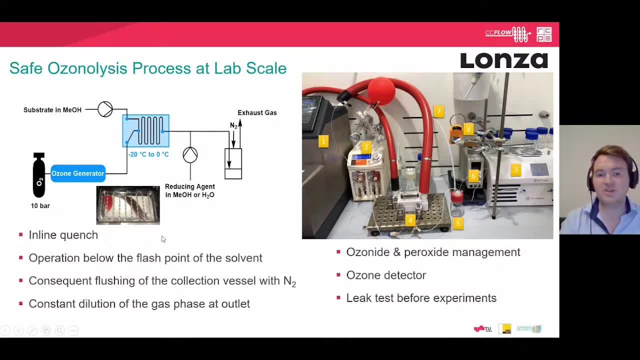 quench is very important to ensure that um we don't see the accumulation of um potentially um exothermic intermediates and explosive environments. we want to try to operate below the flash point of the solvent to ensure that there's not any chance um of explosions and 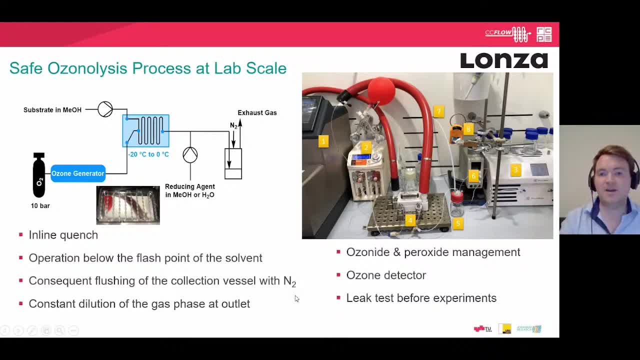 then also we want to keep diluting the outlet vessel with nitrogen gas, And then also- here you can see- the ozone detector, And then one thing that we always did before each experiment is to perform a leak test with an inert gas to ensure that the system. 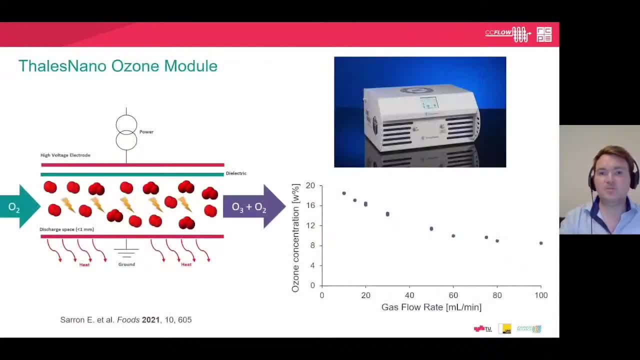 was sealed. So in terms of the Thales Nano system that we were using, so this can operate between 100 milliliters per minute down to one milliliter per minute And it can generate ozone concentrations between approximately 18 weight percent and about eight to nine. 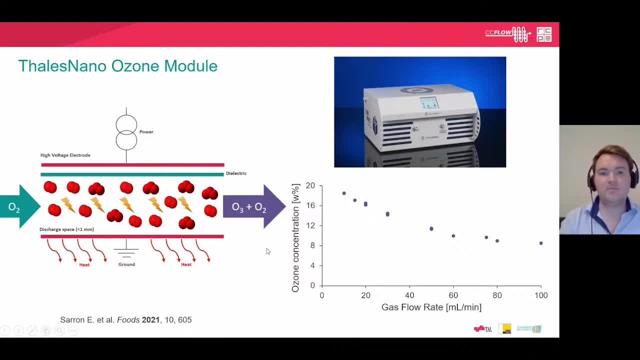 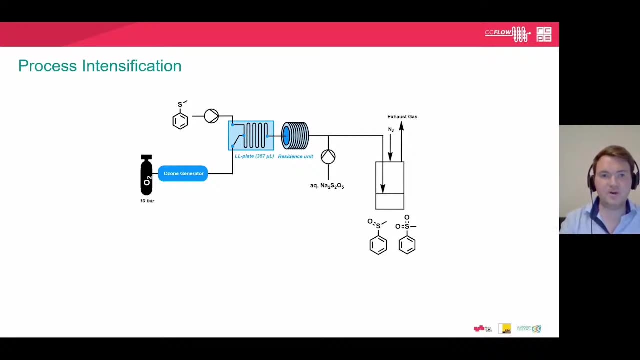 weight percent, depending on the flow rate that you use, And it can operate up to a pressure of five to six bar. So the first system that we looked at was the. So the first system that we looked at was the, the ozonolysis of thioanisole, and this can form our desired product, and then also the over. 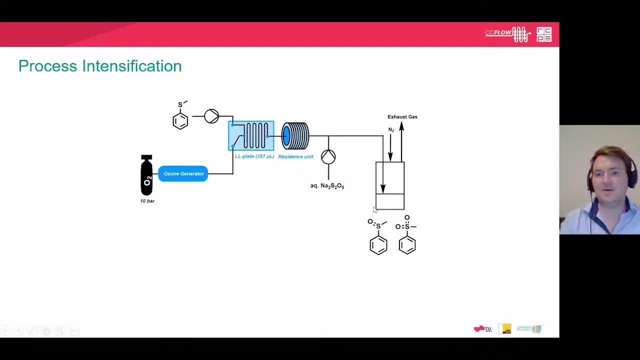 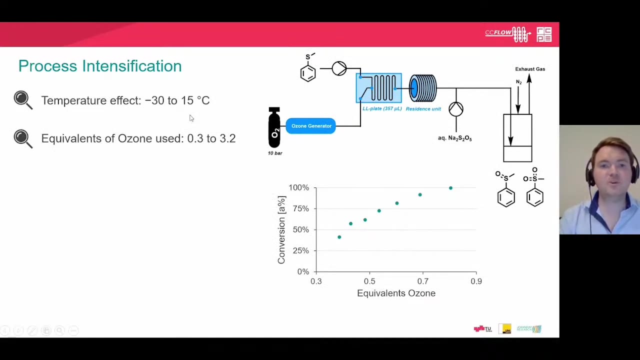 reaction to our side product as well. So we looked at a number of different parameters. so we looked at temperature to see the influence that had. we looked at a wide range of ozone equivalents used, as you can see on the right hand side, as you would expect, with increase in. 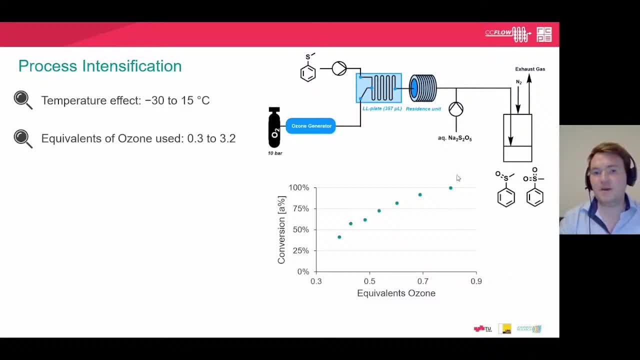 equivalents, then you have higher conversions. One thing that's interesting is you see high conversion even below one equivalent, which indicates that it's probably a radical mechanism that's occurring within the system. We also looked at gas flow rates, along with liquid flow rates to look at. 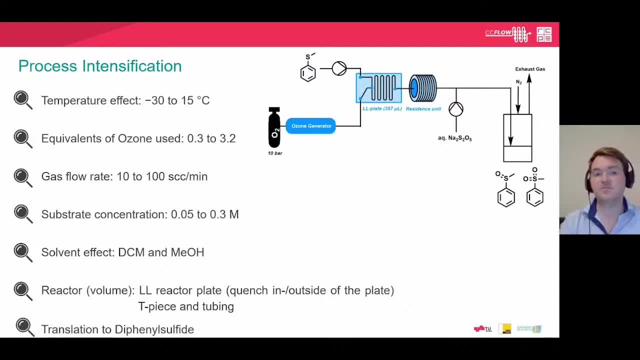 the resonance time that was necessary within the system. we looked at different substrate concentrations, we looked at two different solvents, both dichloromethane and also methanol, and then we also investigated the reaction within a reactor plate, and then also just using t-piece and tubing, We also applied the same conditions. 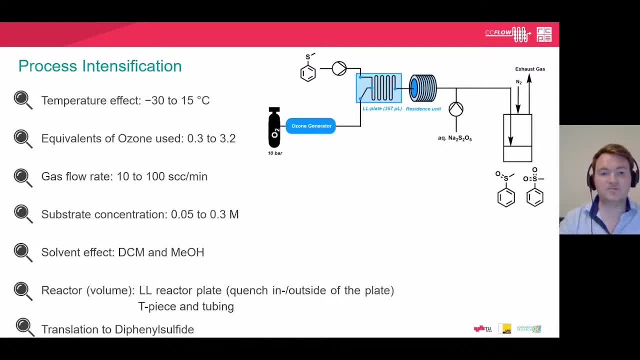 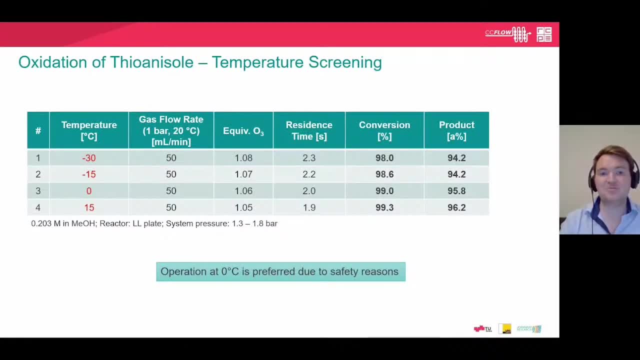 we identified for the ozonolysis of diphenyl sulfide. So in terms of temperature, what's interesting is that temperature doesn't really have an influence in terms of the reaction performance. So at minus 30 we see 94 percent area percent of our product, and then at 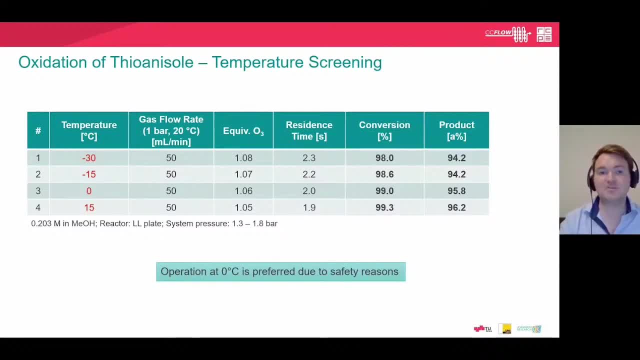 15 degrees we see about 96 percent of our product. So we decided, in terms of our focus, to look at 0 degrees celsius and then also, in terms of our long run, 0 degrees celsius, because then this is operating below the flash point of our solvent. 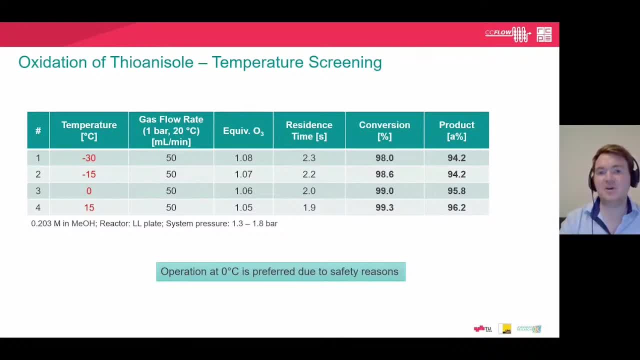 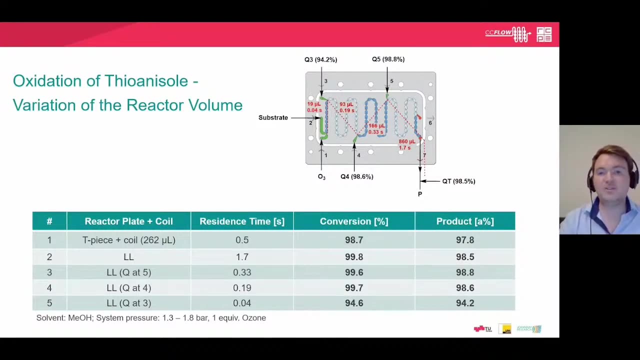 And then, as you can see, here we're only just using a slight excess of ozone and our resonance time is relatively short, of only around two seconds. So looking at the reactor volume and the and the mixing and the influence that that has. so for our first experiment we just tried it using a simple t-piece and a short coil. 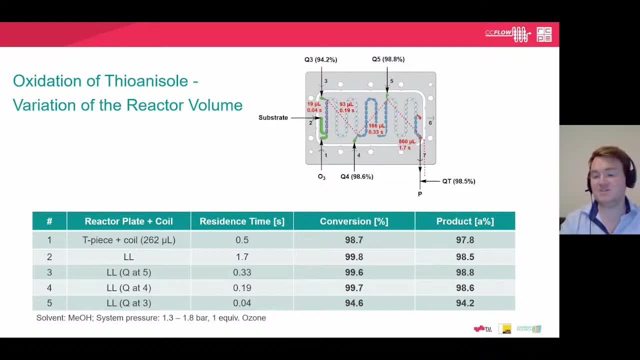 at half a second resonance time, and what's fantastic is that, as you can see, you see high conversion and high product formation. So the thing that this shows is that clearly, at this scale, it works very well within a t-piece and then also when we take the flow plate and we 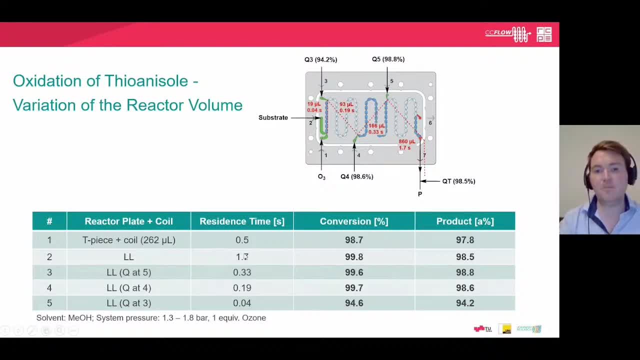 look at different reactor volumes here and different resonance times. So at 1.7 seconds within the flow plate, then we see very high conversion and then a slightly marginally better area percent for our product. and then as we reduce the reactor volume by using different quench inlets, then you see that you also achieve very high conversion. 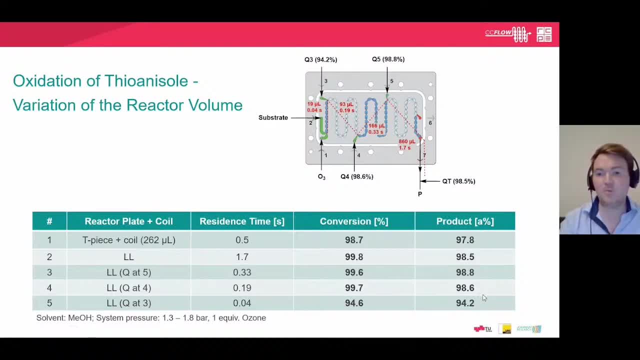 and comparable area percent. It's only when we go to very short resonance time, so quenching within the first corner, at q3 within the flow plate, that then we start to see a drop in conversion and product yield, and so it shows that even within a short time. So in terms of scalability, 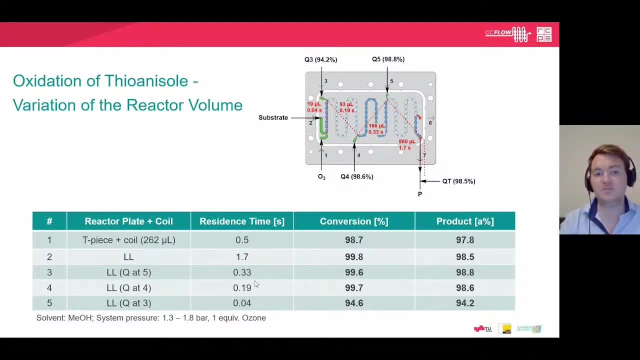 even though, at this scale, the t-piece and coil perform similar to the flow plate, as if this was to be scaled up, then can the same mixing and thermal management be achieved within a two piece and a coil? and the answer is probably not so, which is why you would then look to 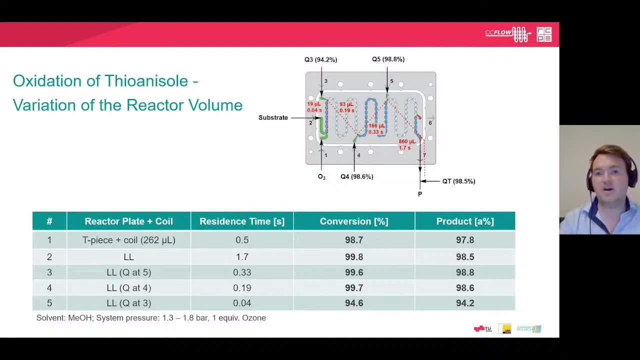 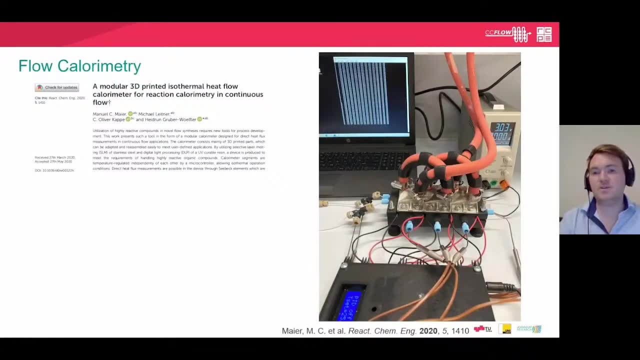 perform it in a, a micro reactor that could give you that, that careful control. So we also looked at the, the transformation within a heat flow continuous flow calorimeter, which was developed in at TU Graz here. So this is a picture of it on the right. So 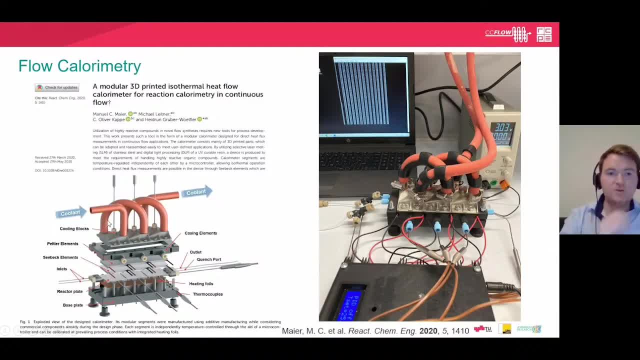 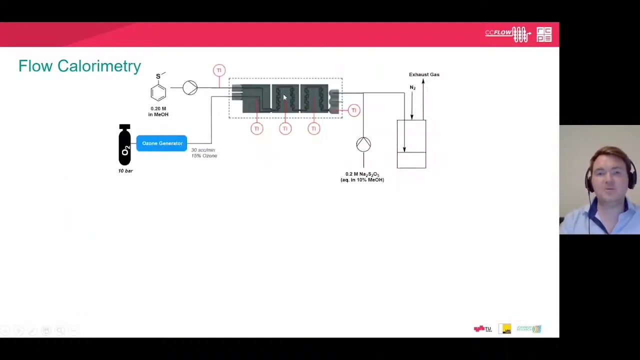 and then an exploded version of it in terms of. so it uses Peltier elements to measure the, the to measure the heat of reaction. So this is a bit more of a detailed schematic in terms of the way that the segments are set up. So within the first one there's the opportunity. 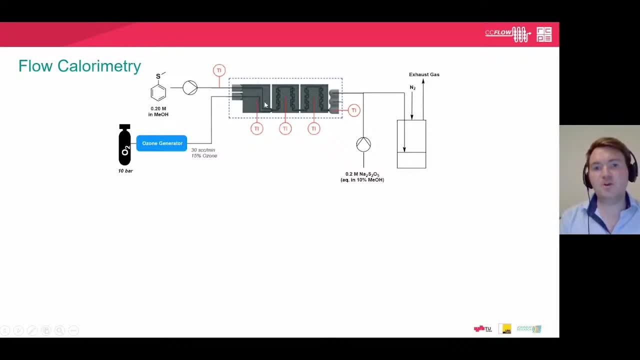 to pre, pre-heat or pre-cool, and then you have two reactor segments where your two feet are mixed, So it's a very similar setup to the flow plate, and then within this, then a very good calibration is necessary. so that you know that, so you can be confident in the measurements that are taking. 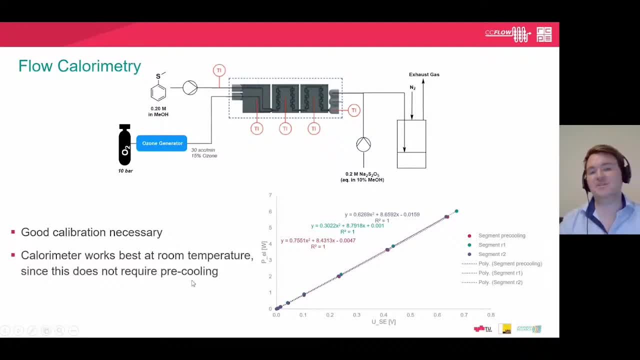 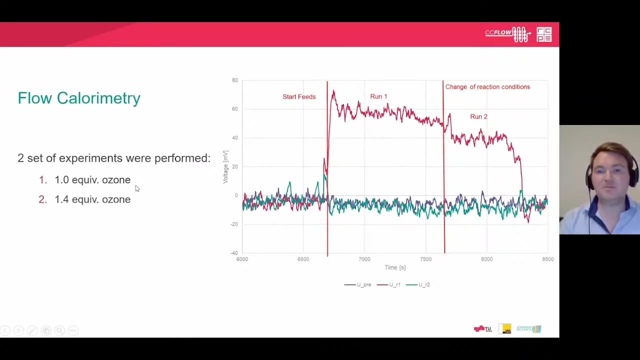 place. So, as I say, the operating a room temperature has a benefit that then you don't need to pre-cool, So it's it's a lot better in terms of that. and so this is. it just shows the results from two separate experiments that were performed, So one equivalent and 1.4 equivalents. 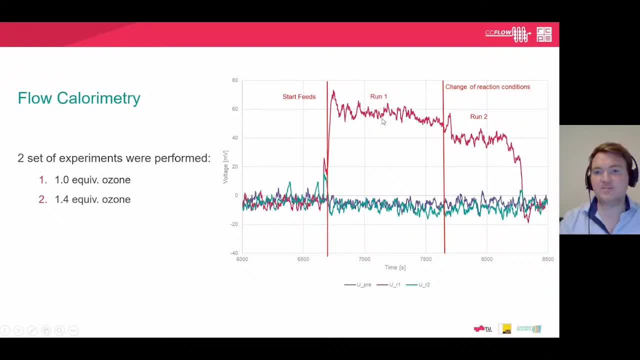 and, as you can see this, this shows the change in voltage. So this is the first set, and then here is the second set, and then, based on this, we could quite confidently measure the heat of reaction. so minus 165 kilojoules per mole, which corresponds to: 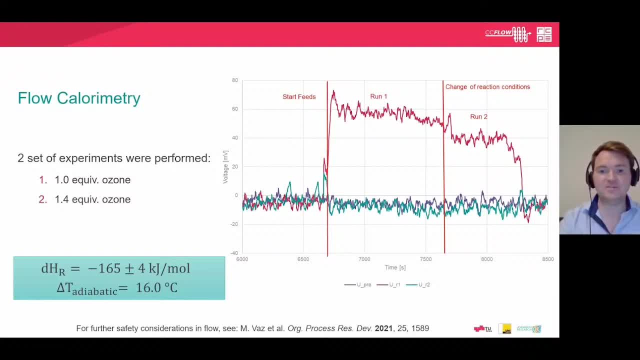 a an adiabatic temperature rise of 16 degrees. In terms of considering safety within ozonolysis reactions, I refer people to this great publication from Corning where they go through a lot of the different considerations that users should consider. I was organised by Quinlan and ICS to generate this table and I can see that I end. Jesus is done, just as the slide should. 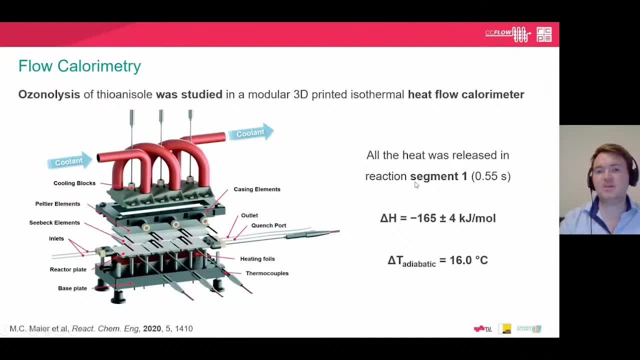 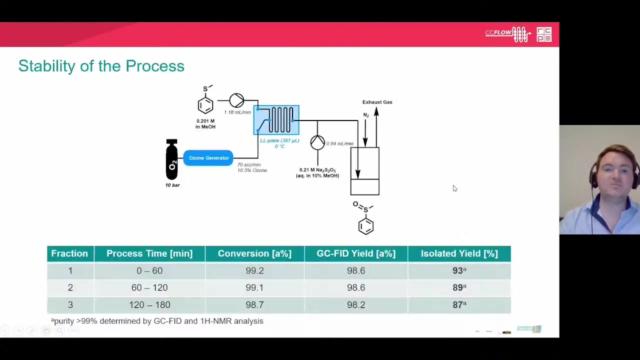 So, yeah, I think the thing that's very interesting within the calorimetry experiments that were done is that we saw that all the heat was released within the first segment, which corresponds to a residence time of 0.5 seconds. So it happens very quickly and there wasn't any heat released in the second segment. 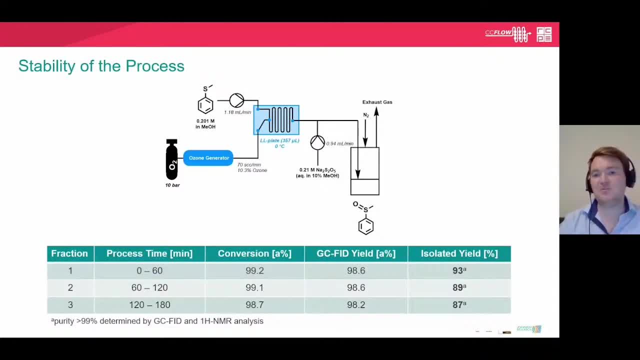 In terms of looking at the stability. we also want to show that not only does it work during our optimisation experiments, that actually we get consistent results as we operate the process for longer. We looked at it over a period of three hours and we saw- based on the optimum conditions. 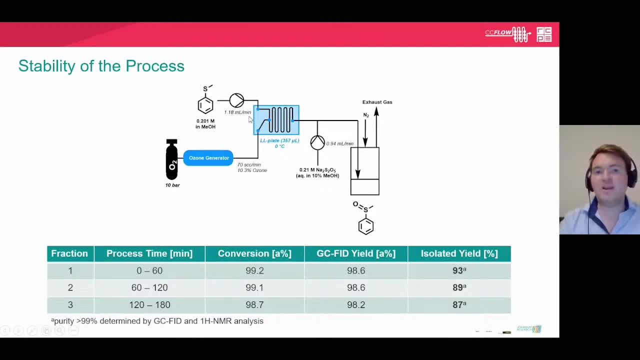 that we were using. so around one millilitre per minute of our liquid feed, 70 millilitres per minute of our ozone in oxygen gas And within the flow plate, and then the quench. we saw very good yields in terms of almost 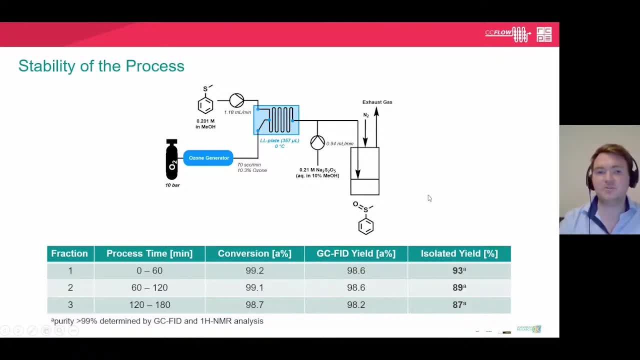 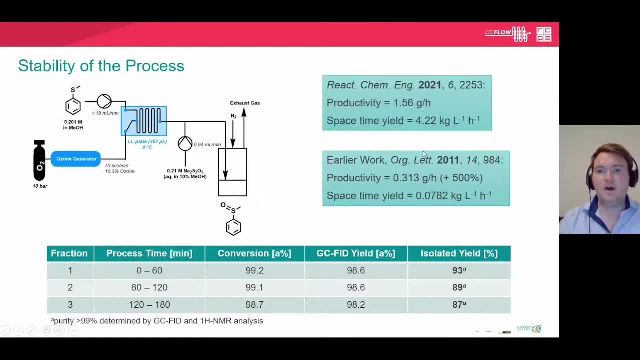 quantitative yields and then, after isolation, close to 90% yield. So it shows that it works for a prolonged period of time, And the thing really to stress here again, coming back to the space-time yields, is that this offers a far better space-time yield compared to earlier work that was done within. 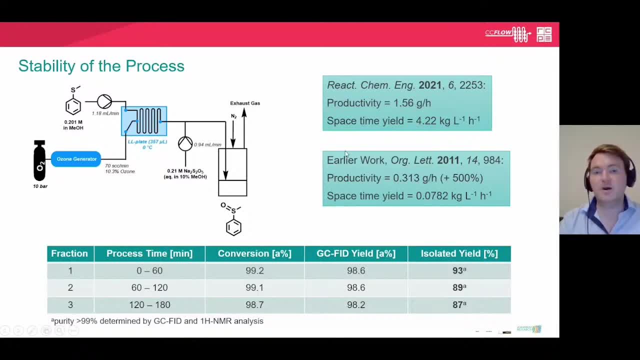 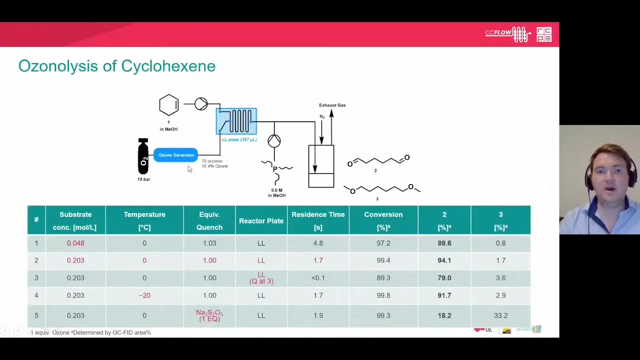 a tubular reactor, And also in terms of the throughput as well, because quite high because of the short residence times that can be achieved within the micro-reactor. Turning to slightly different chemistry, in terms of the ozonolysis of cyclohexene using 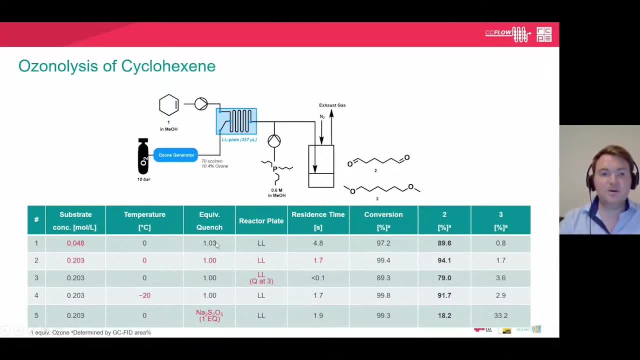 so with similar conditions as for thioanisole. So we looked at a low concentration and a long residence time and saw that you could get 90% of the desired bisaldehyde And then even at higher concentrations at a shorter residence time. then this led to. 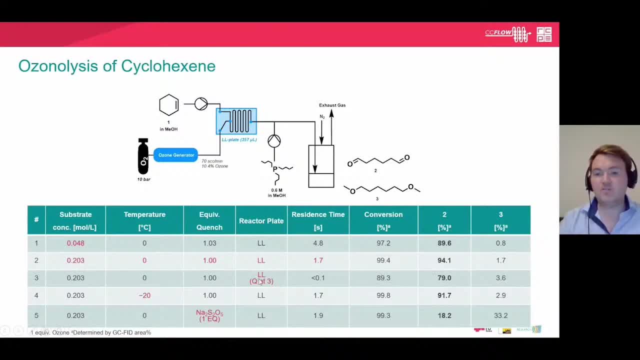 an increase And then when we had the quench at an earlier inlet, then we saw that again in a similar manner to the thioanisole, that there was a drop in conversion and then also a drop in yield as well. 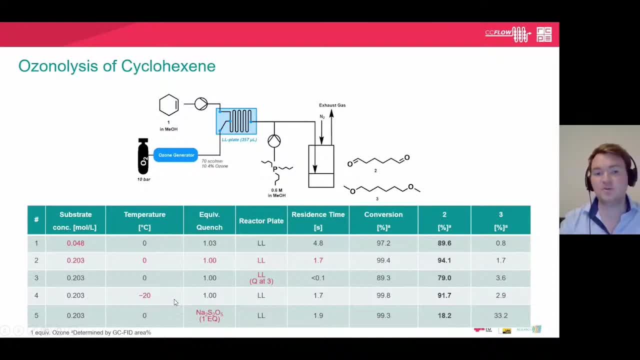 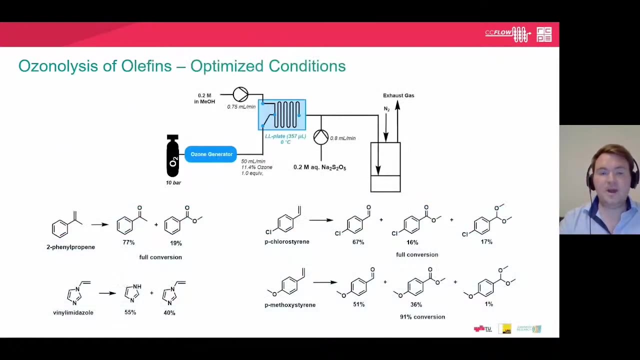 And then at lower temperatures. this provided no improvement, so it's great that we can operate this process at zero degrees. And then when we changed the quench, then we saw that there was a big drop in our desired product. And then we also applied these conditions to look at different substrates using methanol. 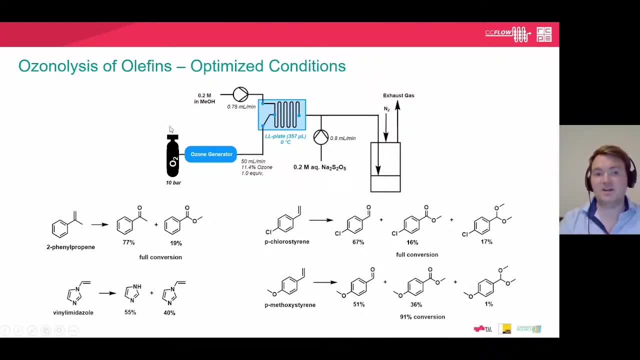 as well. We also looked at the substrates in dichloroamines. We also looked at methane as well, whereby we saw an improvement. So just looking at the methanol example, so as you can probably imagine, you do see the esters formed for these substrates, and then also the acetyls as well. 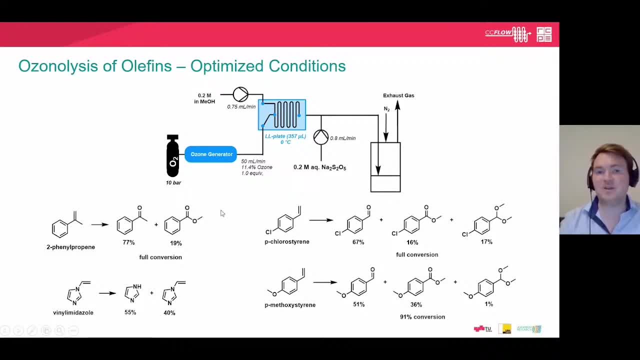 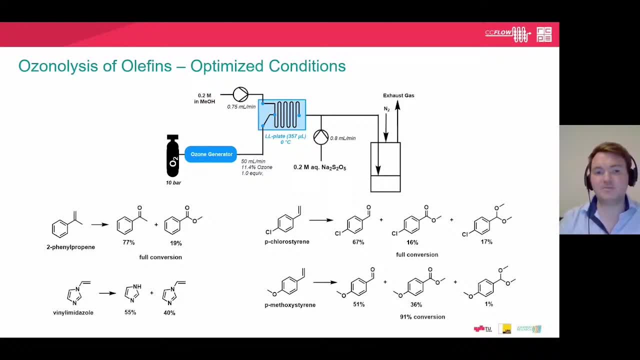 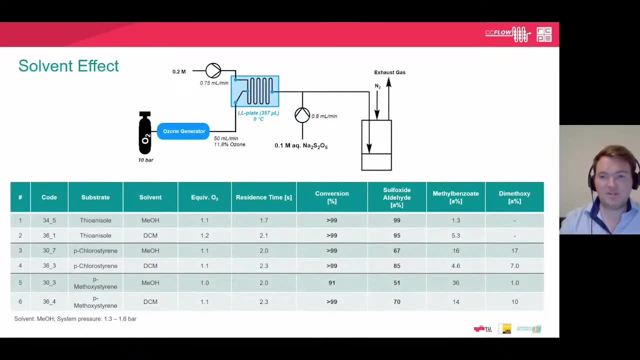 And, as they say, using dichloromethane led to slight improvement with all of these yields as well. but this is not showing So here we can see the improvements that we saw with dichloromethane. so in here, so with 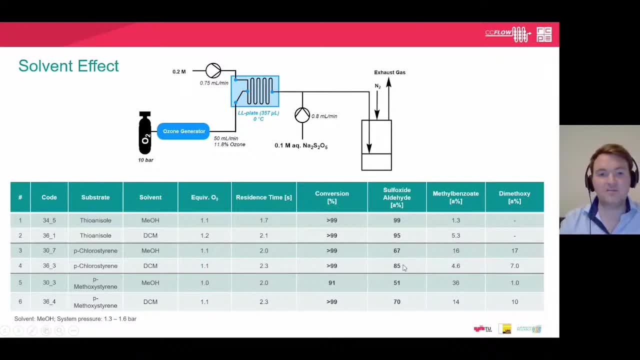 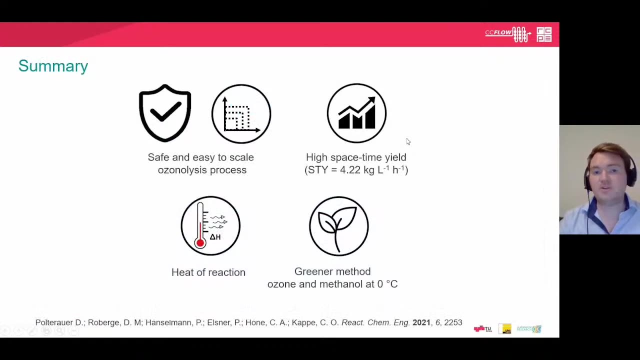 pyrochlorous styrene, so here, 67 to 85, and then again with paramethoxystyrene, again from 50 to 70, so it could further improve our desired product. So as an overview, so I hope I've shown that we can use continuous flow. 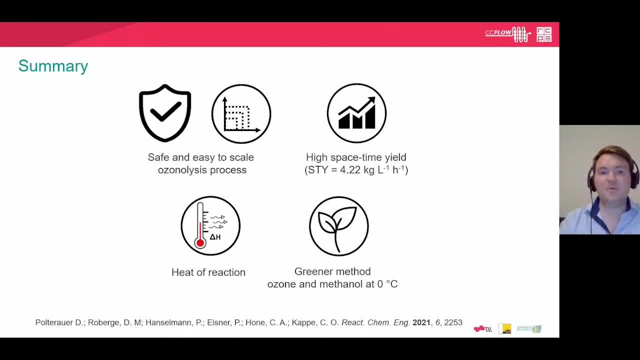 technologies to safely operate these types of processes, and also it gives us the opportunity to take these processes and scale them up. High space time yields can be achieved with this type of process because of the short residence times that are possible. I also showed you that we used a 3D. 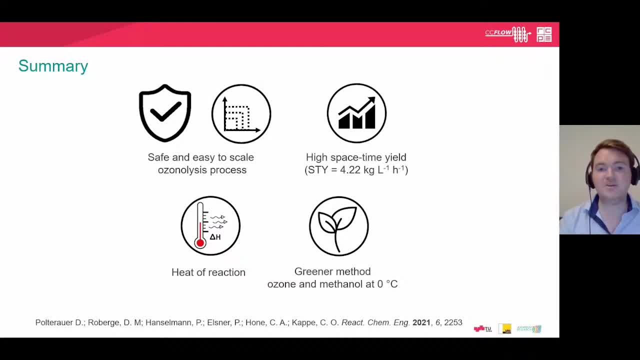 printed heat flow Continuous flow calorimeter from our colleagues at TU Grax to measure the heat of reaction for these, for this type of transformation, and also in terms of the benefit that methanol might have over dichloromethane in terms of providing a greener method, as we saw with the last examples. 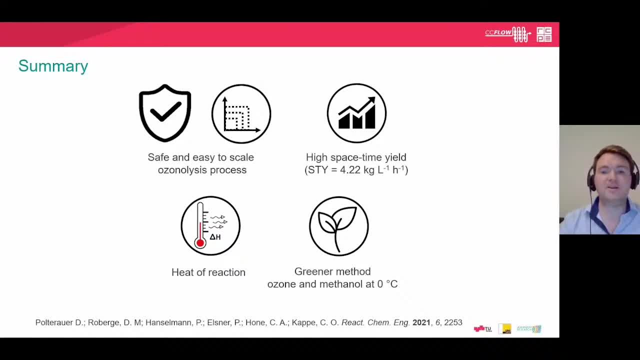 that dichloromethane can sometimes give us a better yield, depending on what product we're after. Actually, if we can use methanol instead and fine-tune towards that, then that's a good thing. That might lead to an improvement. so you can read about the research that I presented within this. 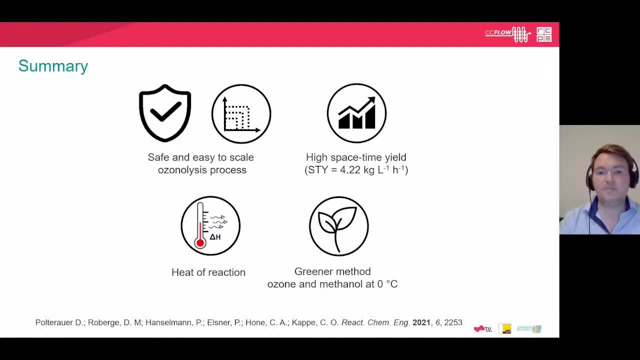 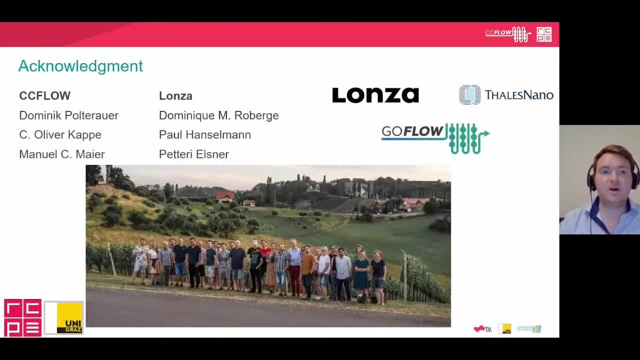 webinar in the paper that's at the bottom and there's more details there as well. So I just would like to acknowledge my colleagues both at CC Flow. so Dominic did the lab work, so he worked hard on that- and performing the analysis as well, My boss and the group leader, Oliver Capper. 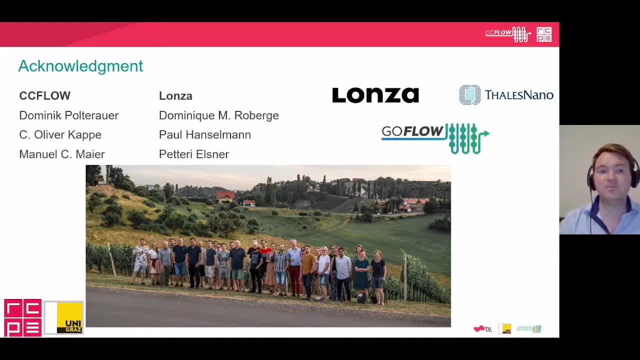 and also Manuel Meyer for their support with the calorimetry experiments. I'd also like to thank Dominic Paul and Pettori from Lonza for their support throughout the project studying the ozone artists reactions, and then also I'd like to thank Thales Nano as well for the opportunity to present the work today and to give this webinar. 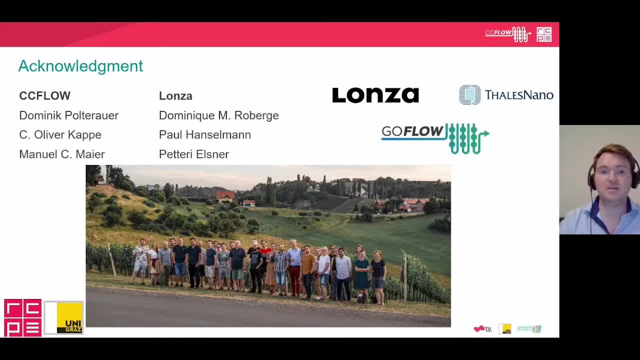 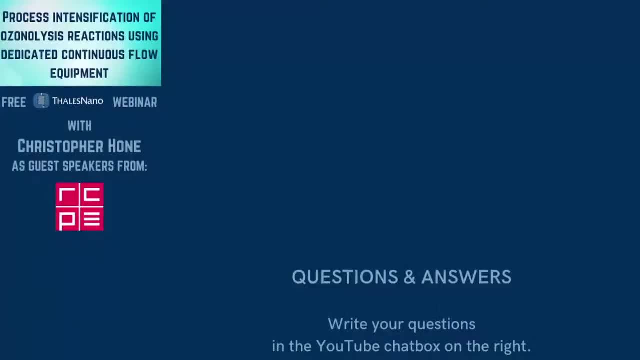 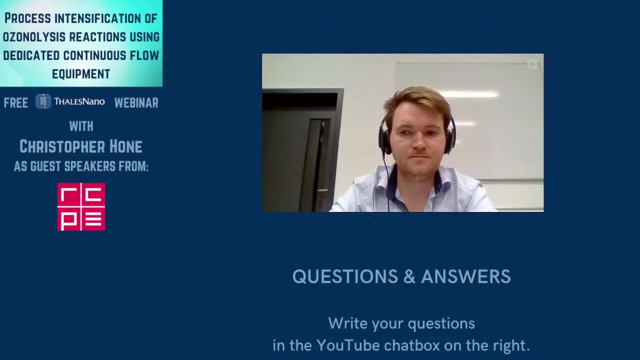 thank you very much and I'm more than happy to take any questions. Thank you, Thank you, Thank you If it's working, So I'll just try again, based on: Yeah, so I've got one question. Have you scaled up any of the reactions you presented? 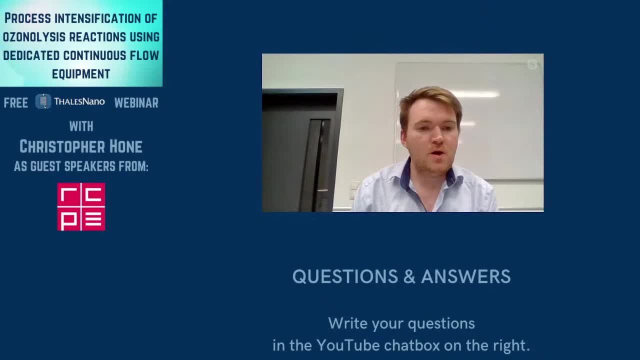 If so, what is the maximum throughput you've achieved? So in this case, we've only operated at the scale you see. So within that, within the flow plate And what we were, we were limited basically by the flow rate that could be produced by the module, because it's a module designed for the lab scale. 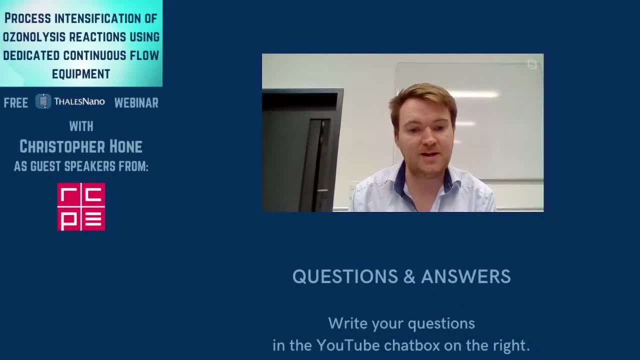 One thing we are looking at now is to get an ozone generator that can achieve a high flow rate, so a prototype. What you're limited by, So, in terms of scaling up, is the pressure drop. So, in terms of what can be achieved across the plate, 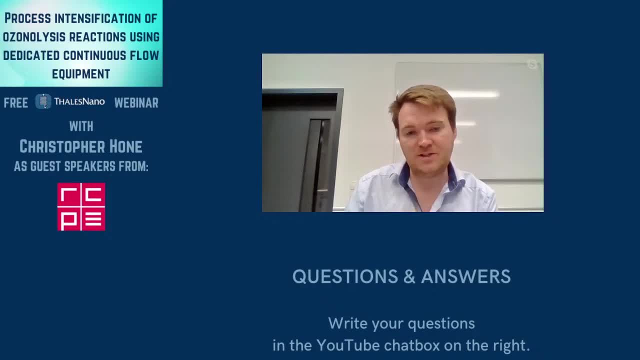 So, if we were to scale up, what we need to be careful of is in terms of making sure that the pressure within the system wasn't too high, Because what you find with a lot of the What you find with a lot of ozone generators is that they're not particularly those designed for. 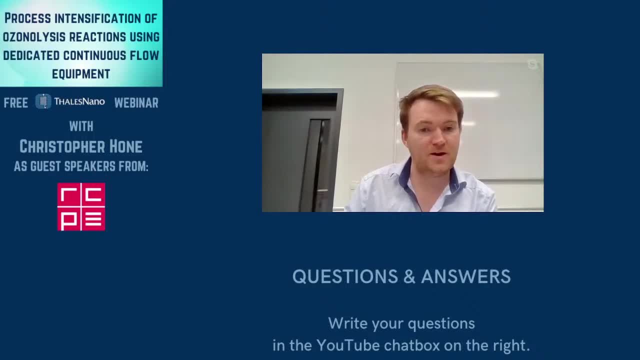 Lab lab scale is that they're not designed to operate at higher pressures. But what we would like to do is to basically demonstrate that this is possible with a high throughput, because what's interesting as well is that we're pretty sure that if you, even even within the same system, even by operating at higher flow rates, we might, we will be able to achieve a slightly higher throughput. 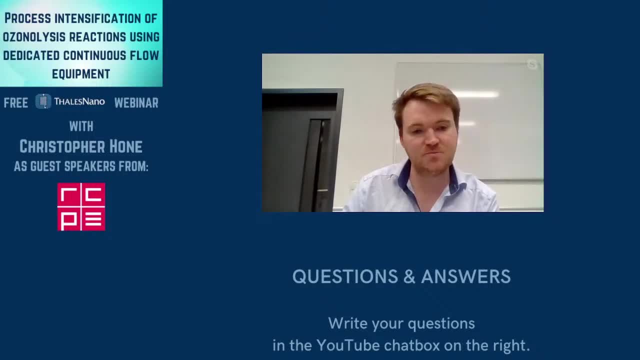 Based on the space, Based on the space time yields that we're achieving, because even within a short zone, within the flow plate we were able to use, we were able to achieve close to full conversion and very good yields. yeah, so I hope that helps to answer your question. so it is something that we're looking at and we 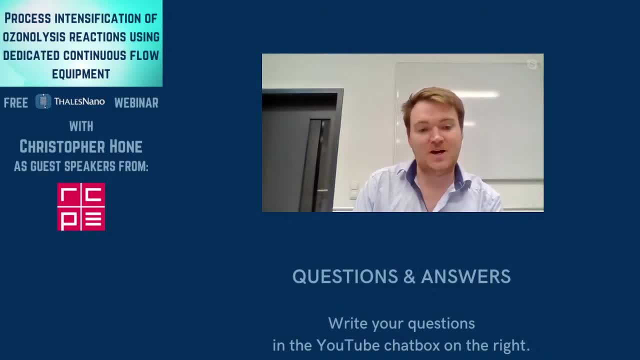 do want to demonstrate at large scales, to demonstrate this idea that you can go from a small flow plate to a larger flow plate and, through maintaining similar heat transfer and mass transfer performance, then you're able to scale up and produce a higher throughput of material. and the vinyl imidazole didn't touch the ring. yeah, so this is this is. this is right. so we saw. 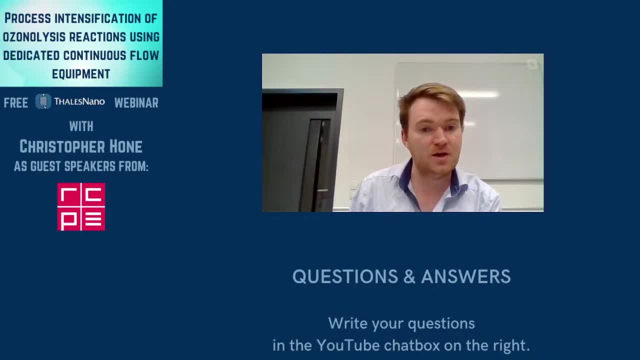 that it was selective to the chemistry that we were trying to do. so we didn't see, we did not detect any, any cleavage of the actual heterocycle itself. so I've also got an another. let me just check to see. so please feel free to write any questions. 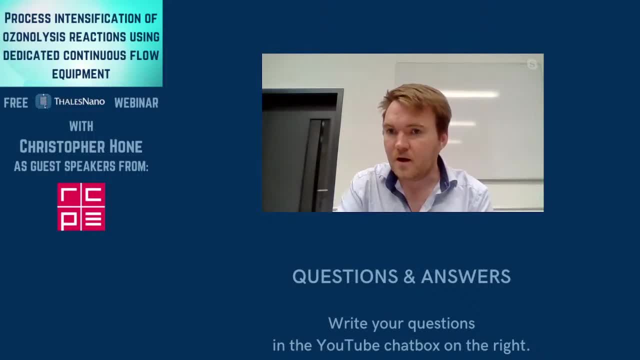 yeah, also thanks for your comments with regards to the the presentation. I really do appreciate it, and please feel free to contact me via email as well if you have any future questions that you think of at a later time, I'd be happy to discuss more and give you. 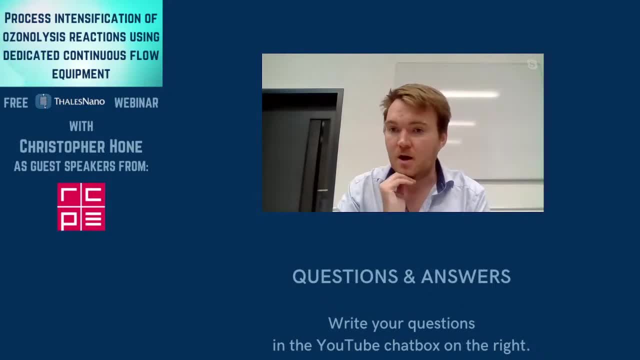 more, more details, and so another question that I've seen as well is that: would it be possible to exclude the quenching step from the flow line and instead collect the product into the quenching liquid? for instance, sodium borohydride is a solid, so it's more difficult to introduce in flow. 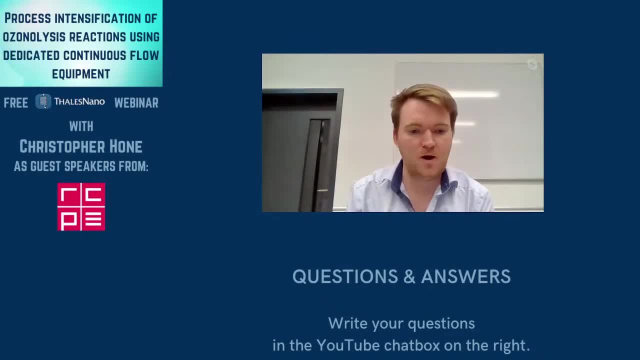 my comments here is that, yeah, in principle, this is possible to do. we, we did it ourselves. in terms of doing the quench within the, within the collection vessel, I would say it needs to be done with care, so safety does need to be considered, for instance, the, the quench. 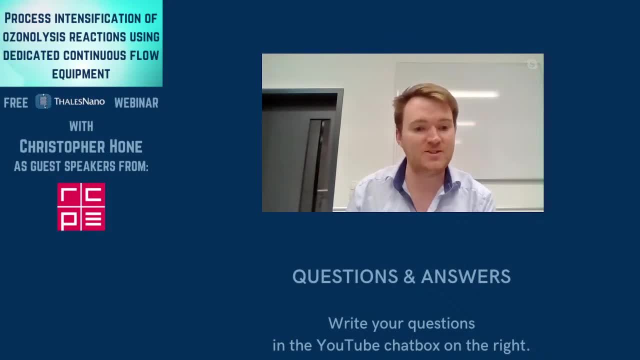 so I the quench of the quench can be more exothermic than actually the ozone analysis reaction itself. so I think, in terms of making sure that it's done- a reaction temperature where you're not going to get a lot of heat generated, you also have to be careful in terms of the the 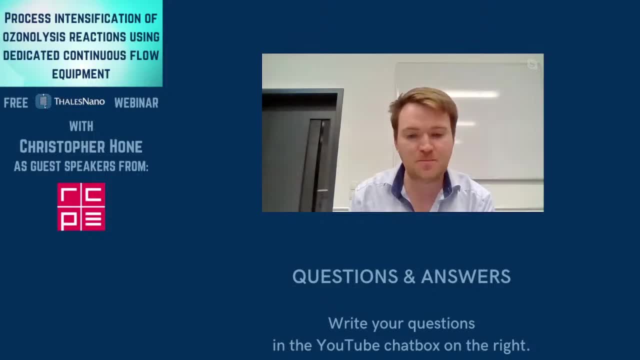 amount of oxygen and ozone present. so it does depend on the scale that you want to operate at, because you don't want these things accumulating so much. so making sure that you're um, you've got your nitrogen line and that there's not so much um, there isn't the accumulation. so one thing also which we looked at is making sure that the 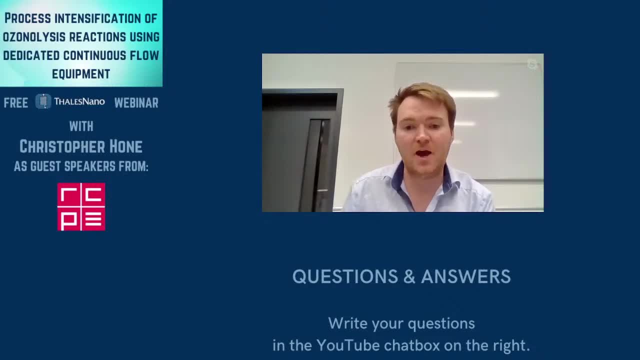 um the ozone um that there isn't too. there is the there isn't too much of an excess of ozone present within the system, and also making sure that if you're only forming small amounts at any one time, then clearly that's a lot safer than when you're operating at large scales as well.